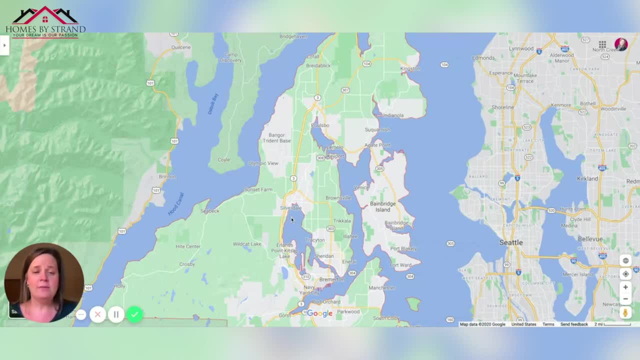 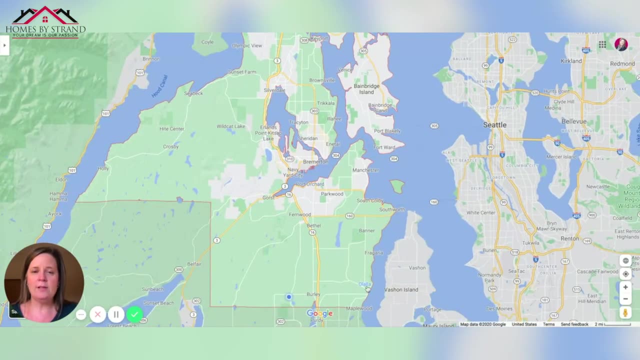 considered the north Kitsap County area. We also have Silverdale, which is central Kitsap, and Bremerton. We have the southern part of Kitsap County which is Port Orchard, all the way down to Beautiful Allala, And you know, I think, the biggest difference between the west side and the east, 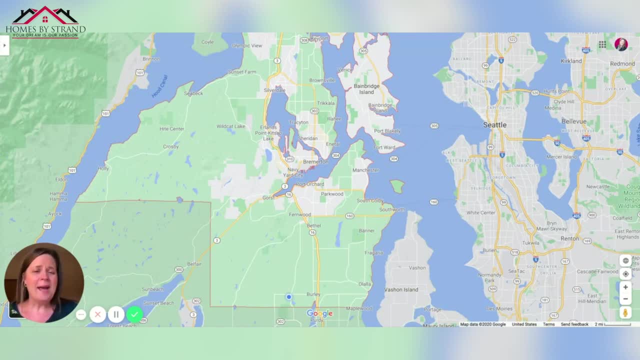 side is the traffic. You know we have some traffic over here, but it's not anything near over in the Seattle or even anything over in the east side area. The incentive for wanting to live in Kitsap County is the fact that you know our houses are still affordable. 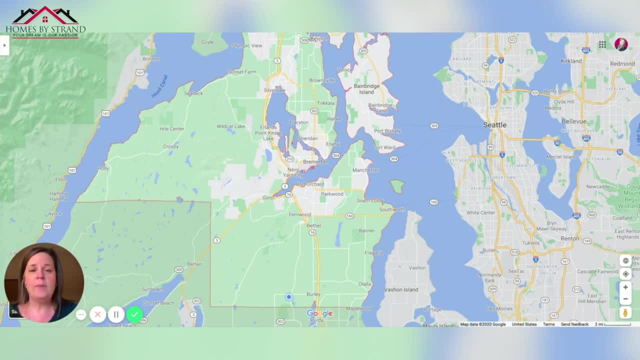 and you're not, you know, forced to buy a home that sits on a postage stamp. So, you know, if you want to live in our little slice of heaven, we have the beautiful over here. We have the Cascade Mountains. over on the east side We have 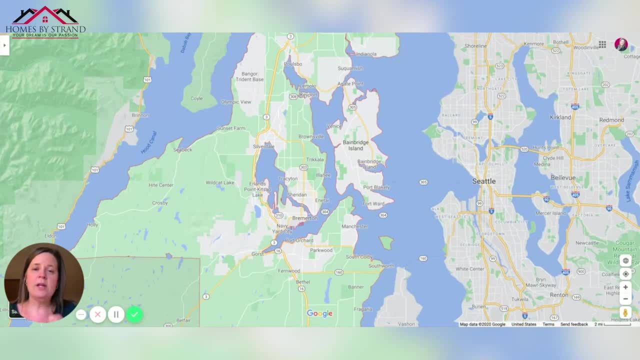 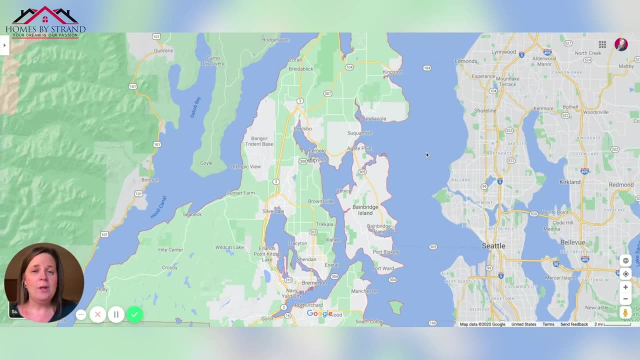 the Olympic Mountains over on the west side, So we just really have a lot to enjoy. So the whole point of the video here again is to talk about. you know, if you want to live in our little slice slice of heaven but maybe your job requires you to commute over to Seattle, we can make that very. 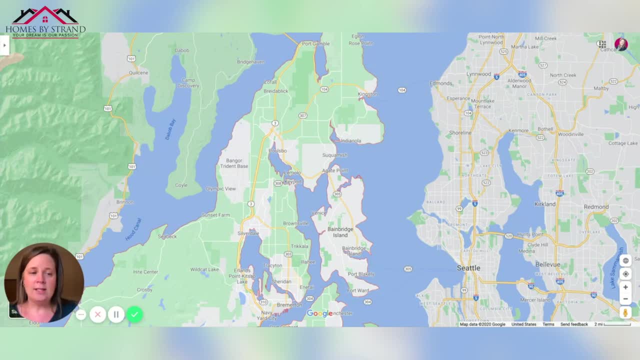 easy. We have several different options as far as the ferry system is concerned to get you over on the north part in Kingston. Kingston and Bremerton both have what's called a fast ferry. It's a foot ferry, And from Kingston into Seattle it's about a 40 minute ferry ride, And from Bremerton into 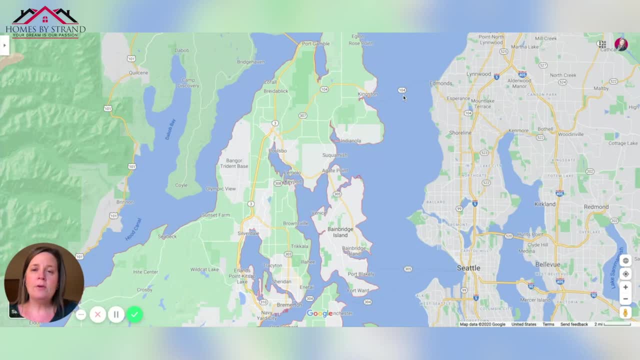 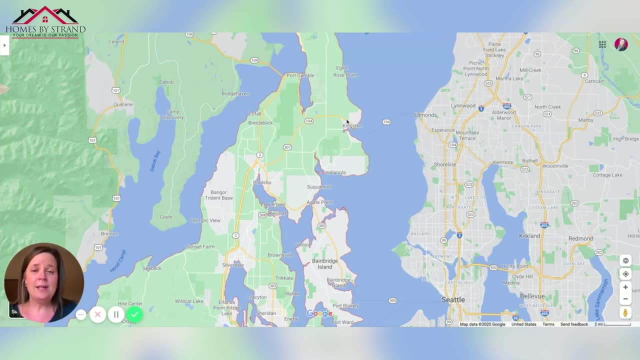 Seattle. it's about a 30 minute ferry ride. Now up here north again. you know a lot of Boeing employees who work up in the north Boeing plant. they like to live over on the west side. here It's, you know, a lot slower paced. There is just more open area And so 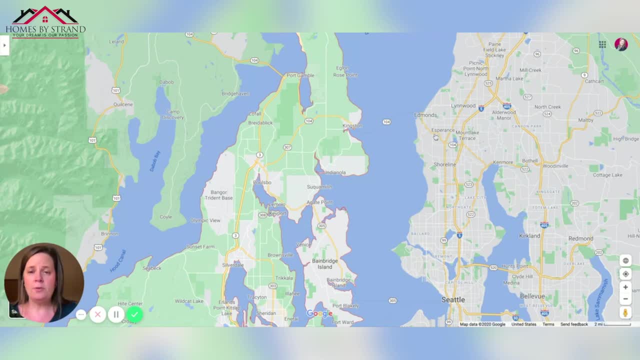 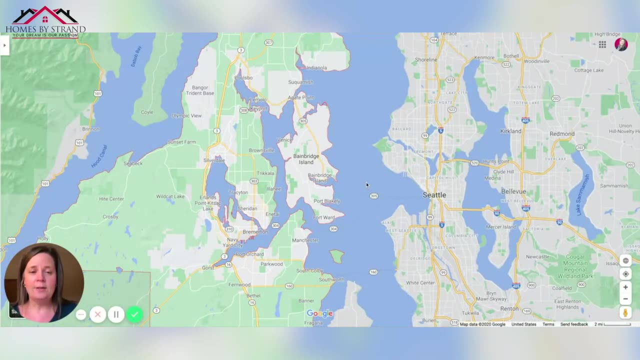 you know, it's a lot easier to get around. So if you're looking for a car ferry, you can take the Kingston Edmonds ferry, which drops you up into the northern part. here We also have a car ferry that leaves from Bainbridge Island. that takes you into downtown Seattle. We also have a ferry from: 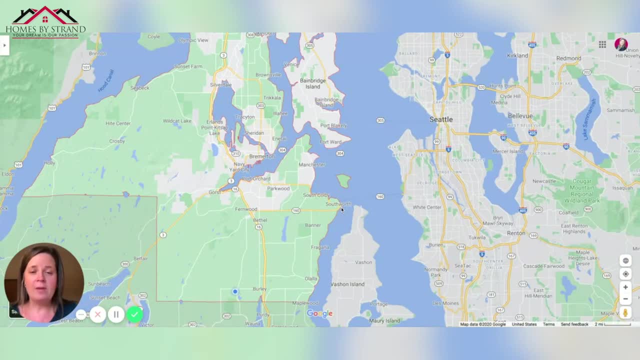 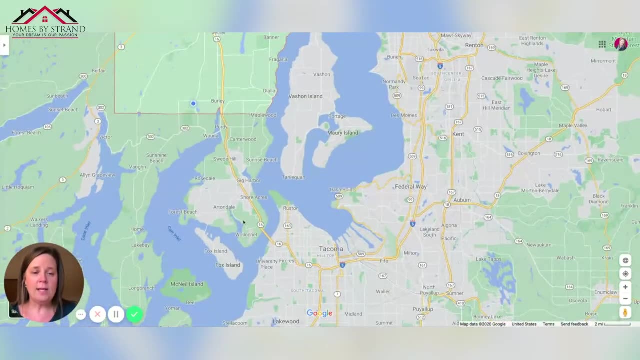 Bremerton a car ferry as well that takes you into downtown Seattle, And then we also have the Southworth ferry here in Port Orchard that will take you into the southern part here. The other option is to take Highway 16, which, again, you know you're going to be dealing with traffic.